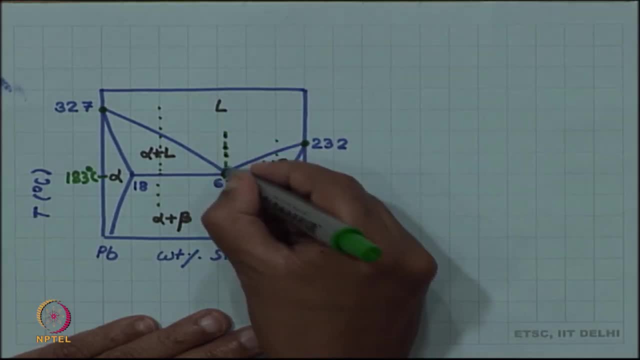 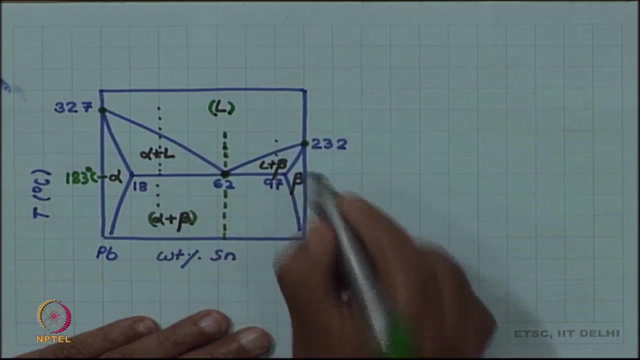 it will remain liquid, Liquid will thermally contract, viscosity will increase, and all that but at 183 degree Celsius. below 183 degree Celsius you see that it is alpha plus beta, and above 183 degree Celsius it is liquid. So the solidification happens at one fixed temperature of 183 degree. 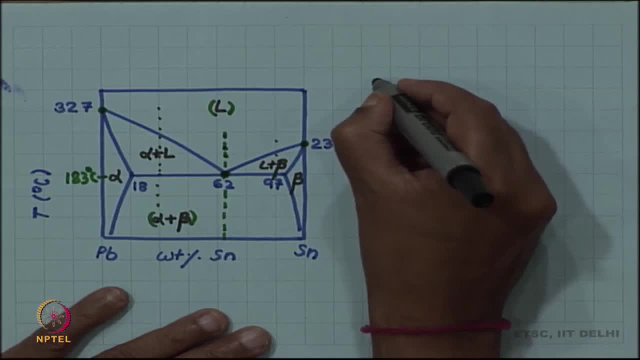 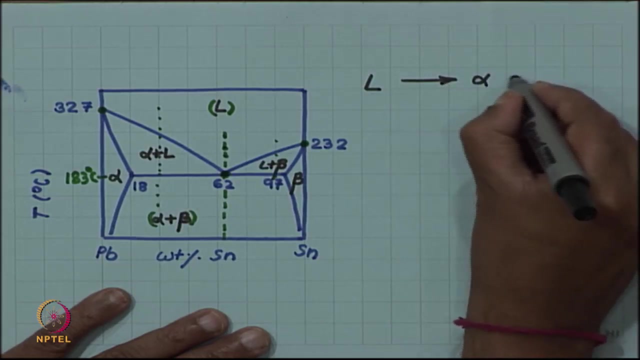 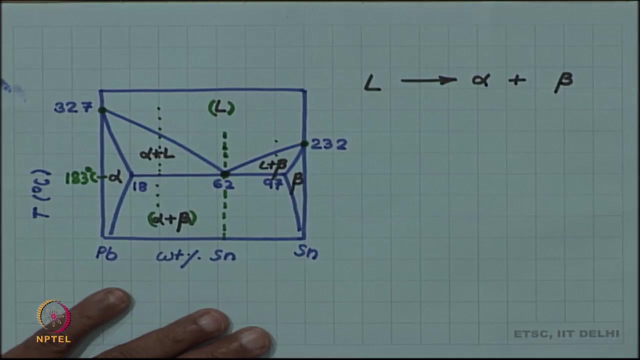 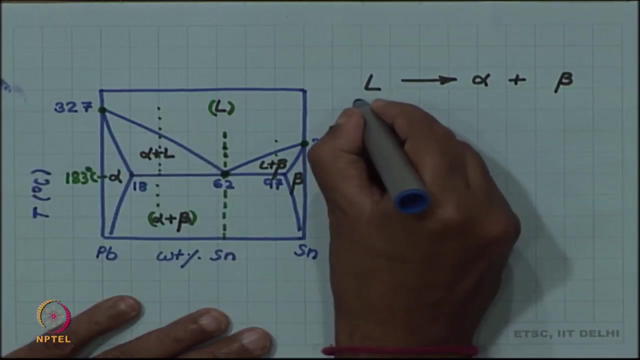 Celsius, just like for a pure element. So on solidification we can write it like a reaction, that on solidification a liquid is undergoing a transformation into alpha plus beta. This liquid is of composition 62, weight percent tin. So I write the composition: 62, units. 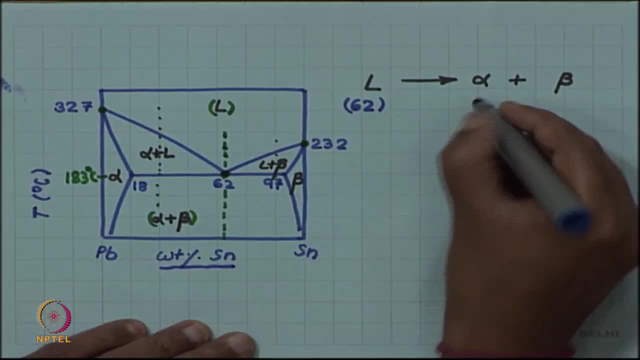 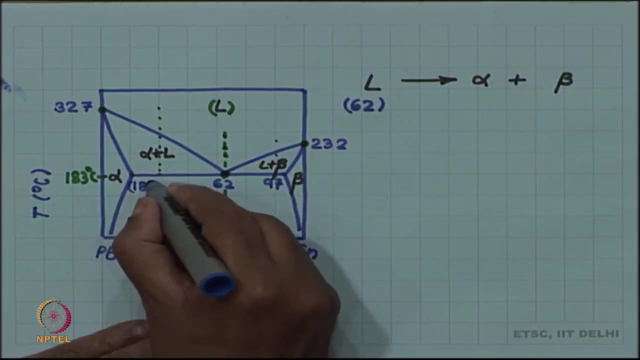 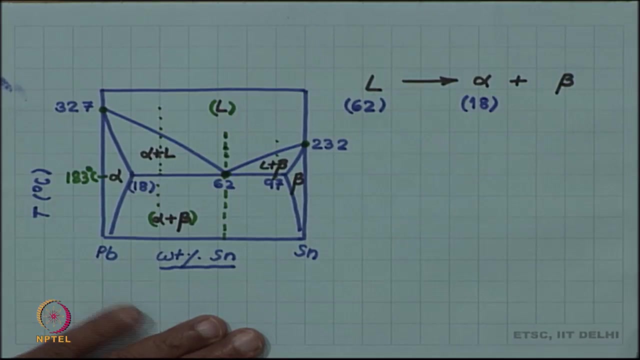 are weight percent tin, So I write the composition 62,. units are weight percent tin, So I write the composition 62,. units are weight percent tin. Alpha which will form by decomposition of this liquid is given by this end composition 18.. So 18 weight percent tin in alpha and 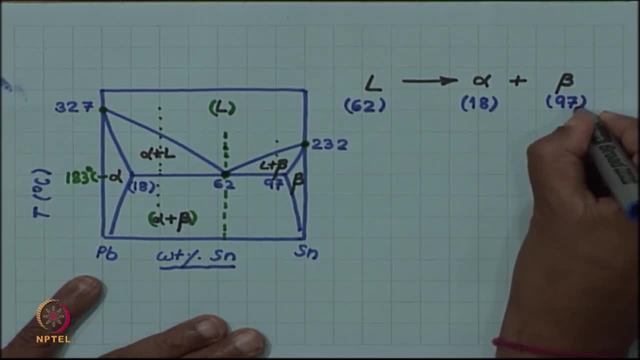 97 weight percent tin in beta. So beta is more or less pure tin with 3 percent lead Alpha is given by this end composition 18.. So 18 weight percent tin in alpha and 97 weight percent tin in beta. So beta is more or less pure tin with 3 percent lead Alpha is given. by this end composition 18.. So 18 weight percent tin in alpha and 97 weight percent tin in beta. So beta is more or less pure tin with 3 percent lead. Alpha is given by this end composition 18.. So beta is more or less pure tin with 3 percent lead. Alpha is given by this end composition 18.. So 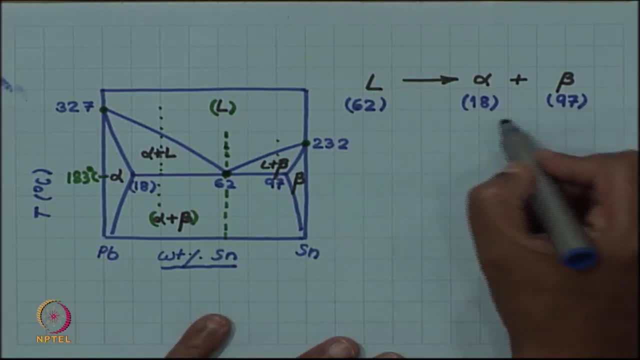 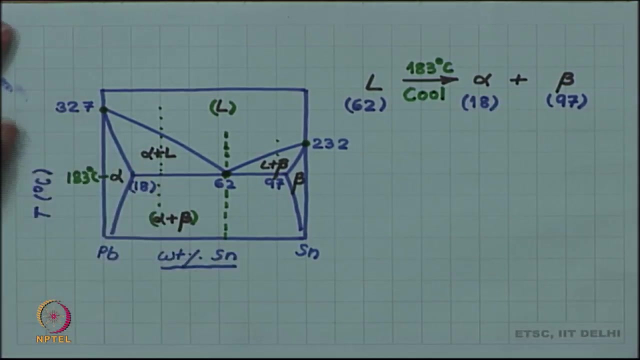 beta is pure lead, but with a significant fraction- 18 percent- of tin in it, And this reaction is happening at 183 degrees Celsius. So I write this over arrow and the direction of the arrow is cooling. the reaction will happen if you cool the liquid. So this: 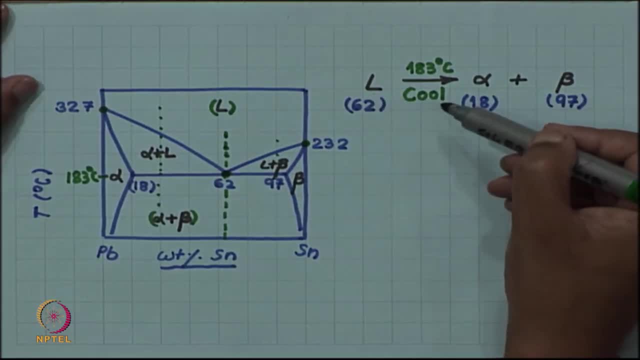 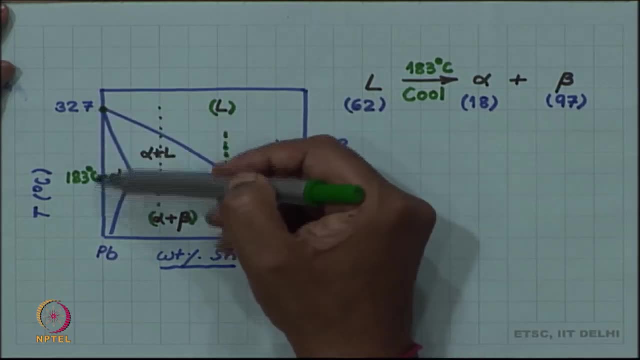 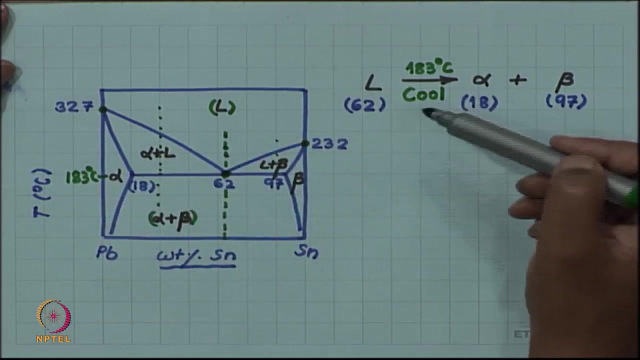 is just like normal solidification, where a liquid, on cooling through the its melting point, solidifies. Only difference is that a normal liquid, like a lead liquid or a tin liquid, will solidify into a single solid phase. a eutectic liquid solidifies into two, a mixture of two different solid phases. 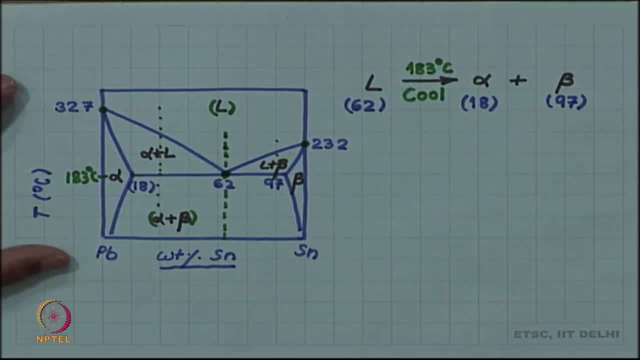 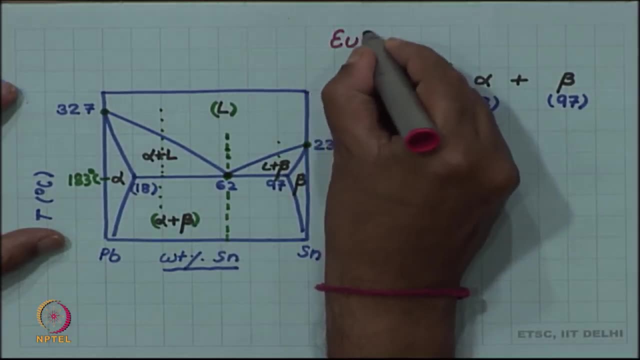 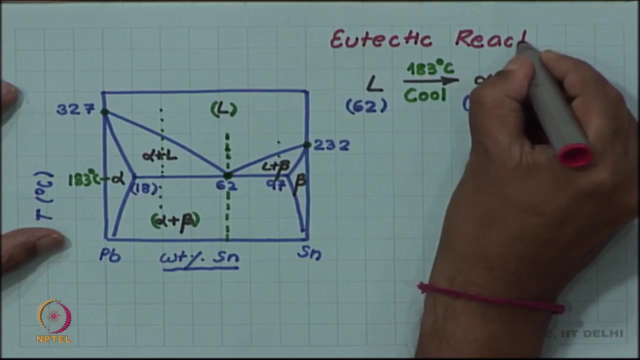 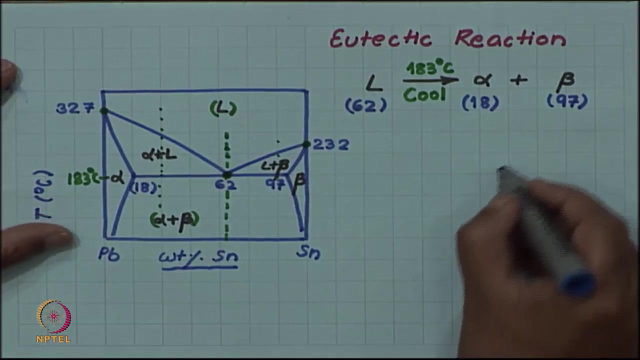 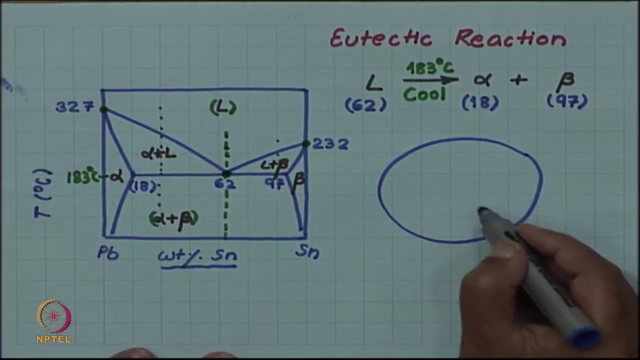 So such a transformation is called a eutectic reaction. So this has been given a name: eutectic reaction. If you think in terms of microstructure, you just try to draw the microstructure. So suppose this was all liquid and you hit at 183 degree Celsius temperature. then the 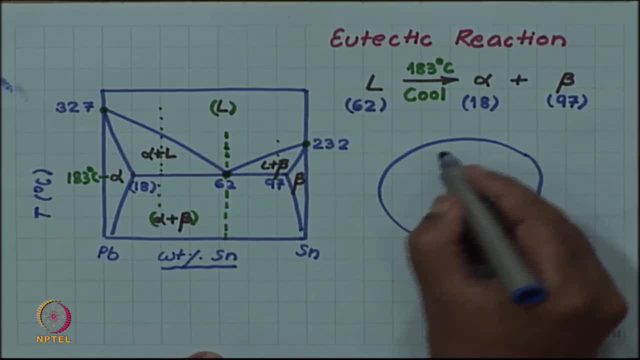 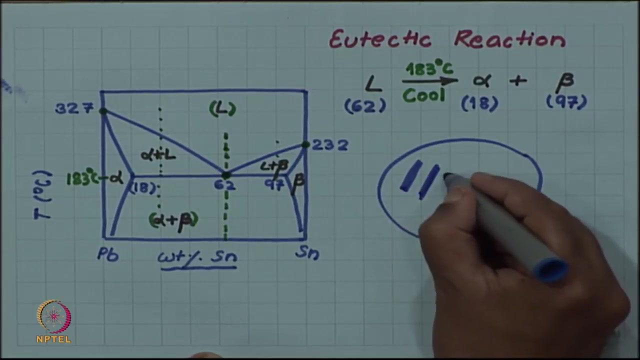 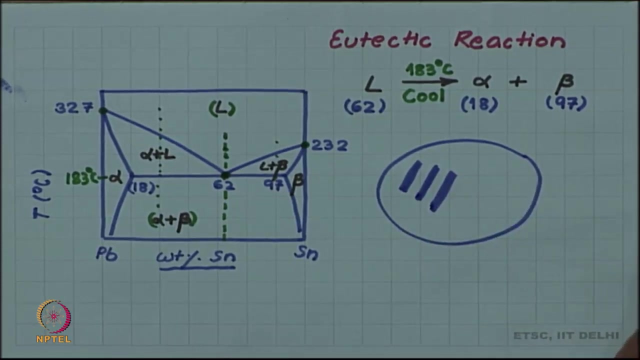 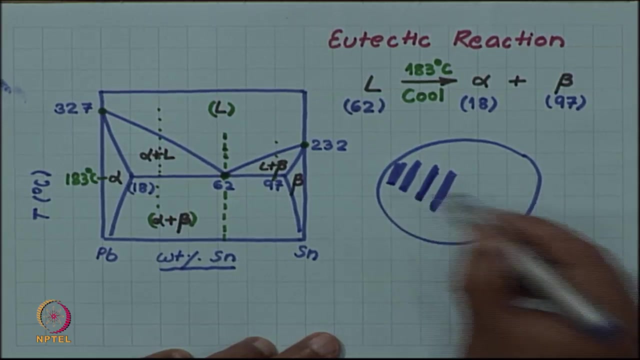 solid phase will start forming and this solid phase will be a mixture of alpha and beta. So let me draw alpha by the, as these blue plates and many eutectic and in case of lead, tin also. So the mixture of the two phases come as alternate plates of alpha and beta. So in 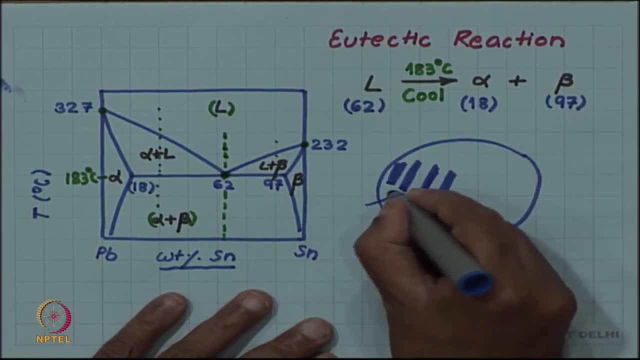 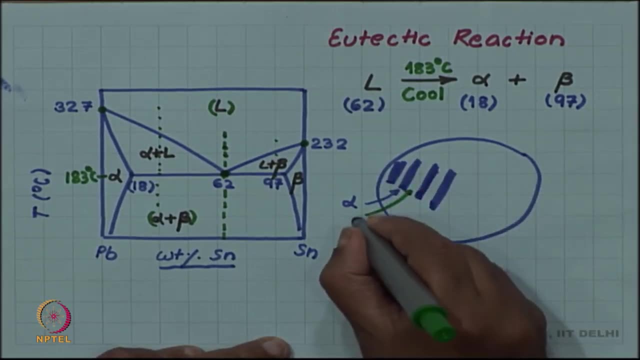 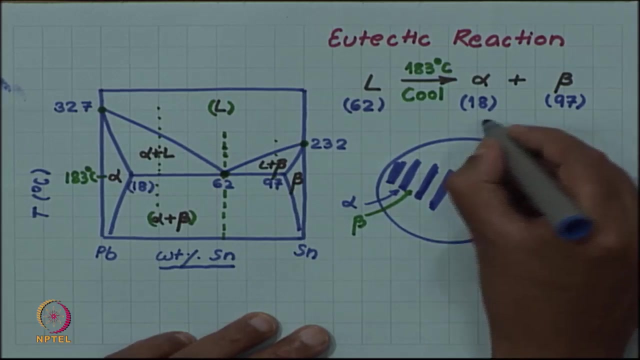 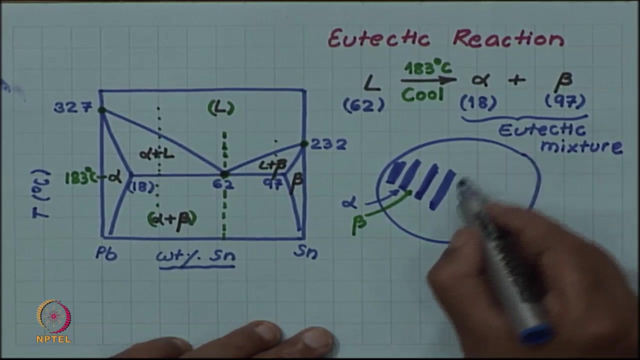 this case, I am representing these plates as alpha and, in between, what I have not colored as beta. So you are forming a eutectic mixture. this is called a eutectic reaction. The product of a eutectic reaction is called a eutectic mixture. and just like you had different 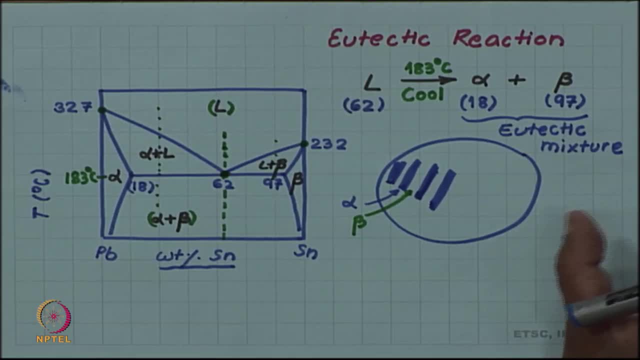 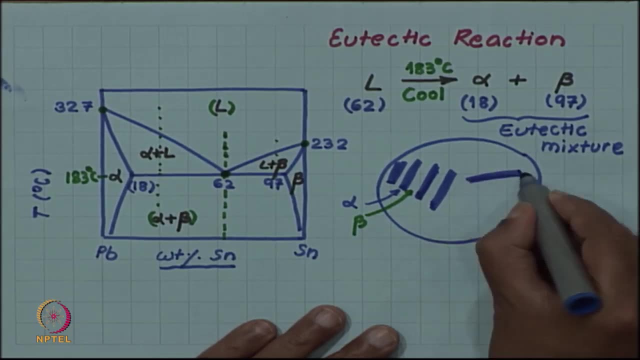 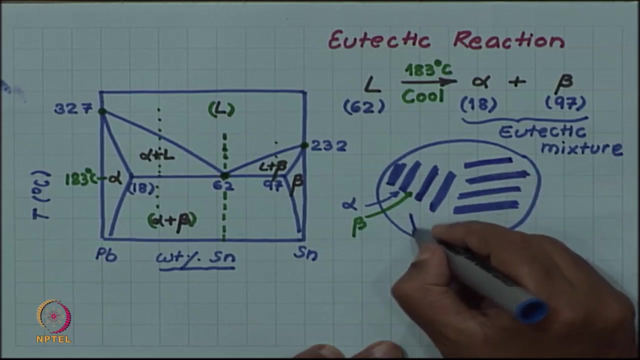 orientation of crystal in an isomorphous system. here also, in different region, the alpha and beta plates will nucleate but they will not have the same orientation. So in some other region of the alloy again alpha and beta plates are there, but they are different orientation. 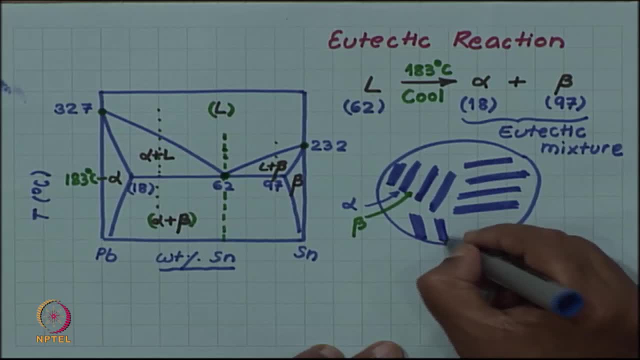 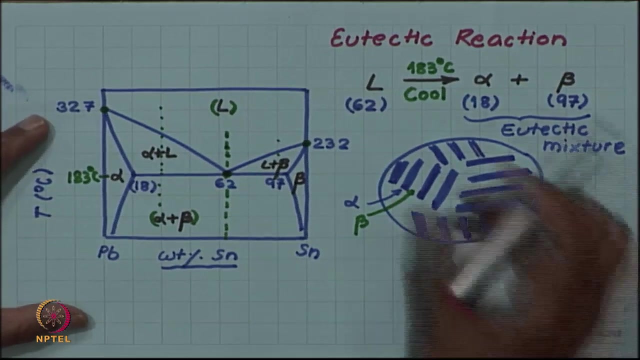 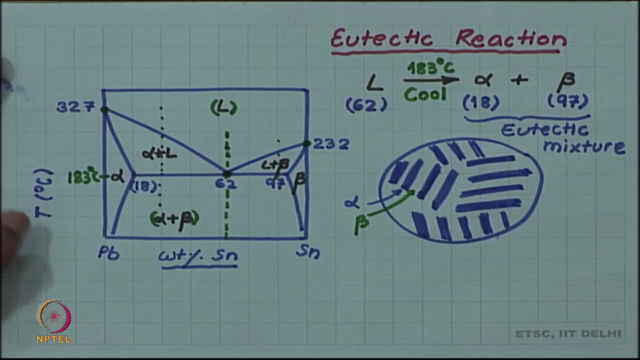 Get another region. you have yet another orientation. Yes, Good, Good, Good. So this is a schematic I have drawn. you can see a real let in microstructure. may be on the web and you will find that, or in a text book you will find a real microstructure. 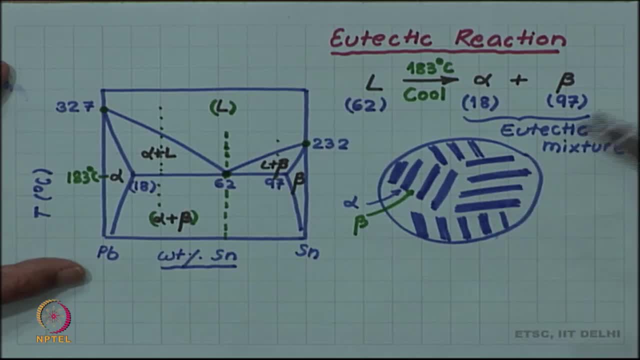 will not exactly look like this because this is a cartoon drawing, But essential feature is that microstructure of eutectic will have alternately alpha and beta phase, because that is the product of liquid transforming through this eutectic reaction. 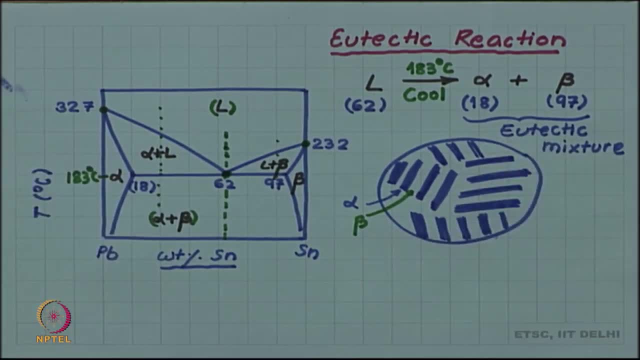 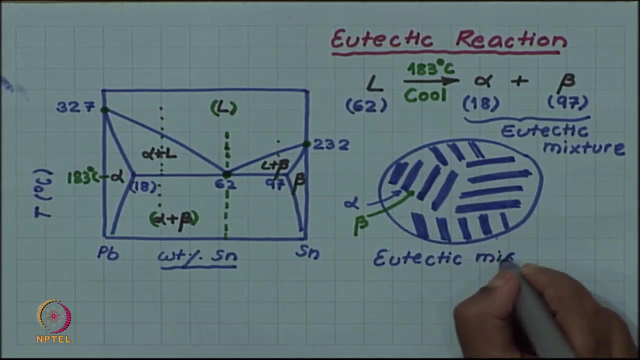 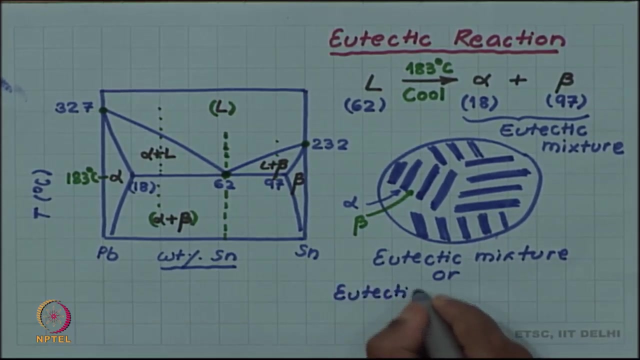 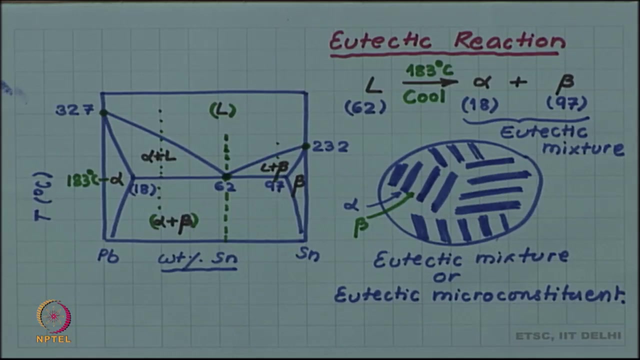 So this is this feature, this microstructure feature is called the eutectic micro constituent or eutectic mixture, eutectic mixture, This eutectic reaction. I will end with the mentioning one point, that this eutectic reaction. 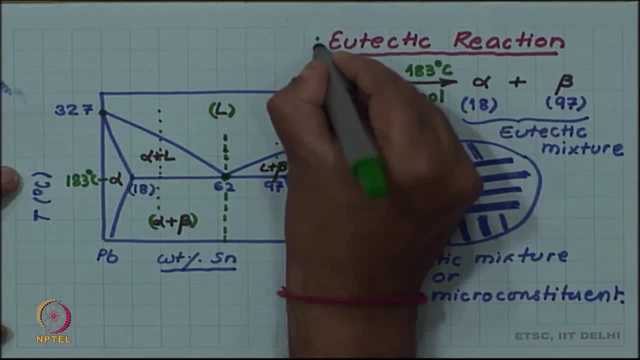 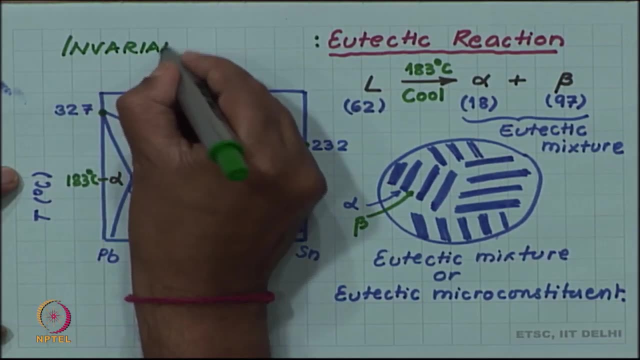 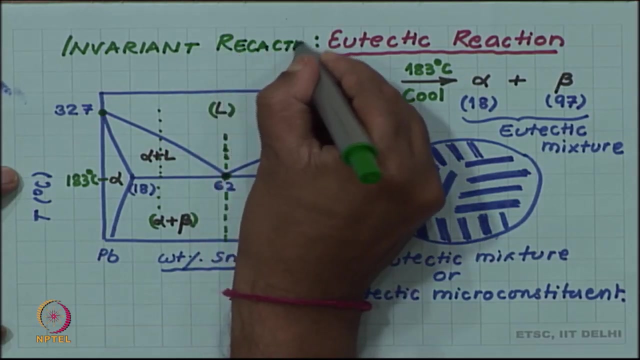 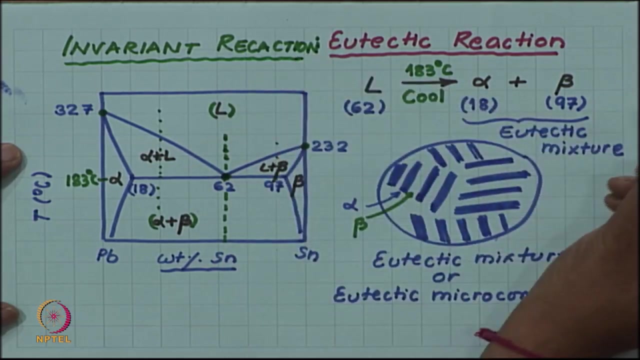 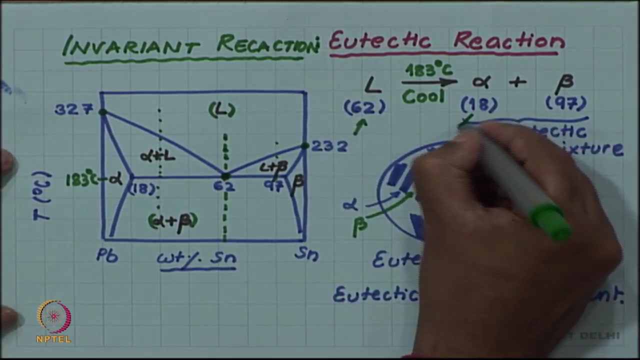 is an example of an invariant reaction. The invariant reaction what it means? that the eutectic reaction happens at fixed composition of the phages. So liquid, in this case liquid, is of 62 weight percent, alpha is 18 weight percent and beta 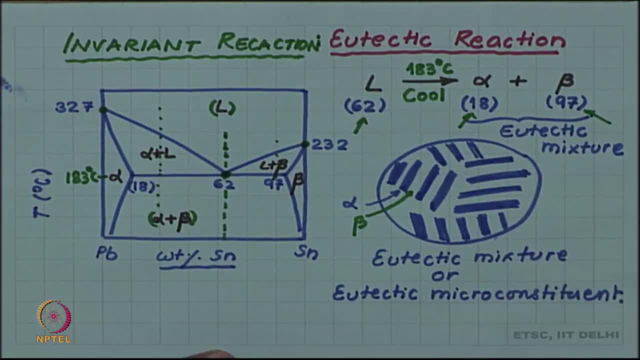 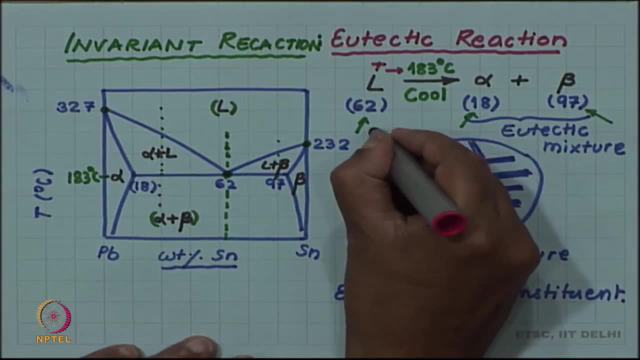 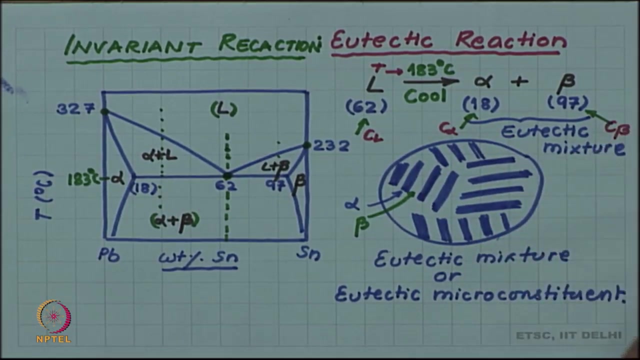 is 97 weight percent at a fixed temperature. So neither the temperature nor the composition of the liquid phase, the alpha phase or the beta phase is a variable when this reaction happens. So since all these, the three compositions and the temperature, is fixed during the invariant reaction, during. 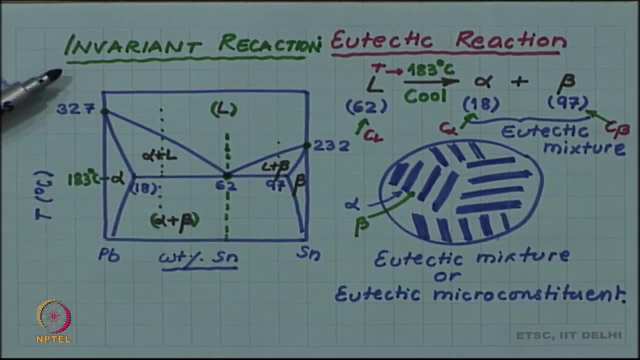 the eutectic reaction. we call such reaction an invariant reaction and eutectic reaction is one example of such reaction. we will have opportunity to look at some other invariant, several other invariant reactions during the this course.